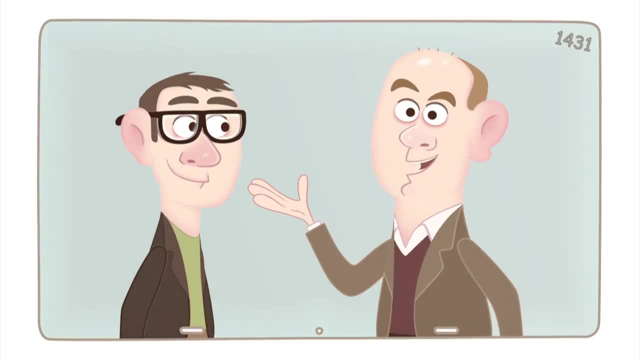 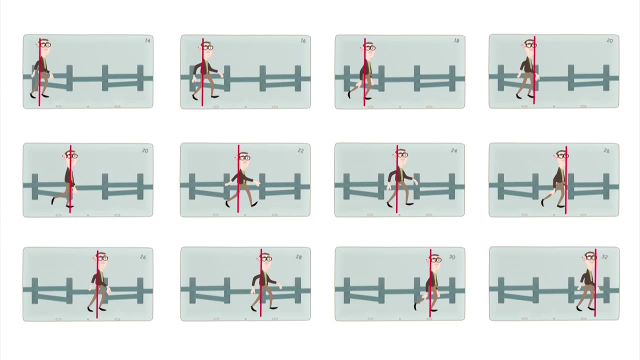 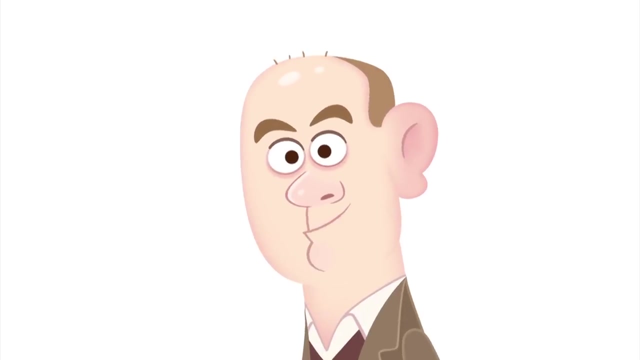 You'll need more panels. More panels, please. Okay, in each panel Andrew's in a slightly different place, so I can see each one records where Andrew is at a different time. That's great, but it would be easier to see what's going on if we could cut out all the hundreds of panels and stack them up like a flipbook. 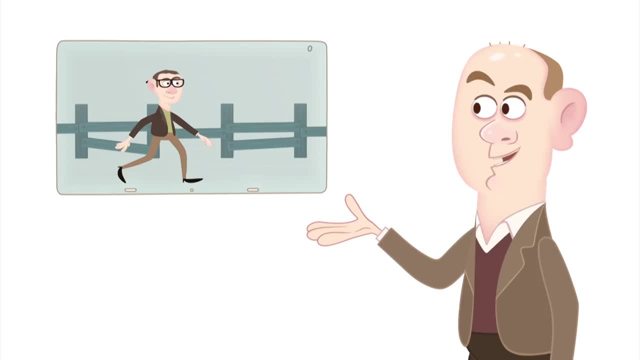 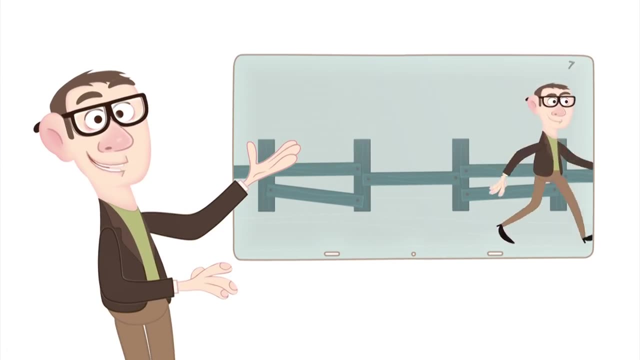 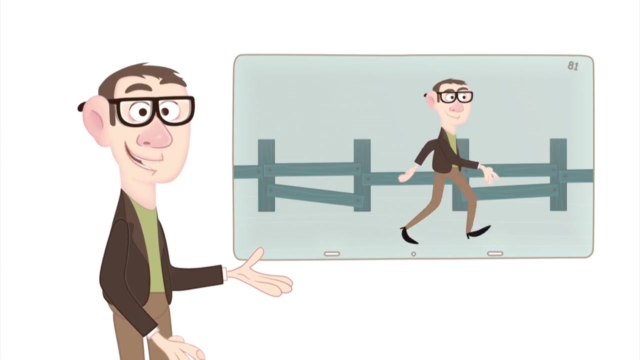 Right Now let's flip through the book so that we can see one panel after another getting through, 24 in every second. See, I told you it was an animation. Now you can see me walking along, Drawing all those panels and putting them into a flipbook is just one way of recording the way I'm moving. 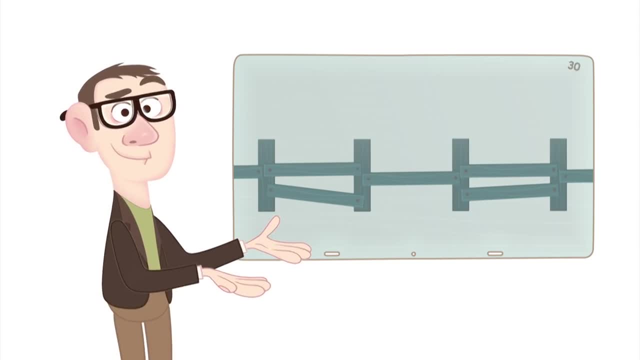 It's how animation or even movies work. As it turns out, at my walking speed it takes two seconds to get past each fence post, and they're spaced four metres apart. So we can calculate my velocity. how fast I'm moving through space is two metres per second. 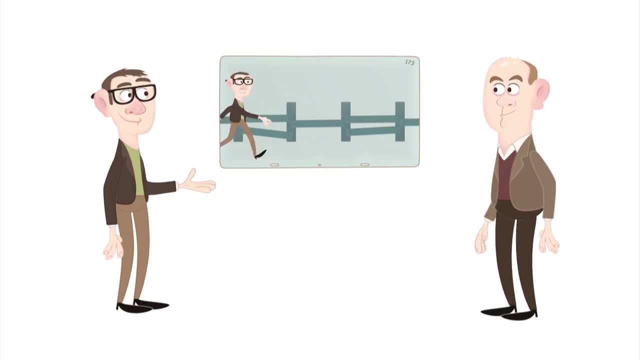 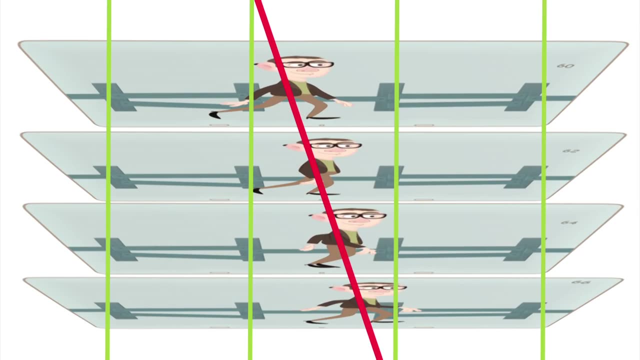 But I could have worked that out from the panels without flipping through them. From the edge of the flipbook you can see all of the copies of the fence posts and all of the copies of Andrew, and he's in a slightly different place in each one. 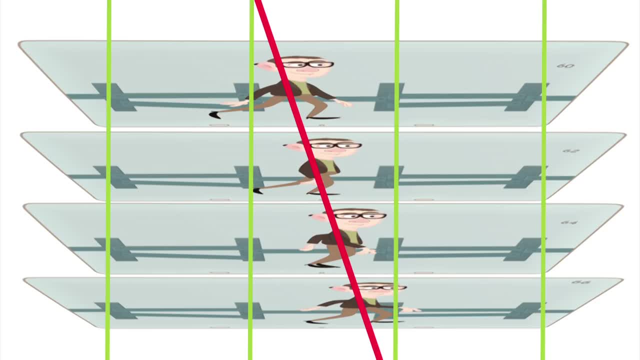 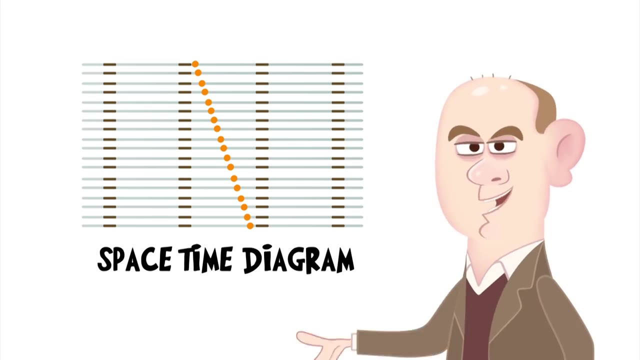 Now we can predict everything that will happen to Andrew when we flip through 24 pages every second, Including his speed of motion. just by looking, No need to flip through at all. The edge of this flipbook is known as a space-time diagram of Andrew's journey through. you guessed it: space and time. 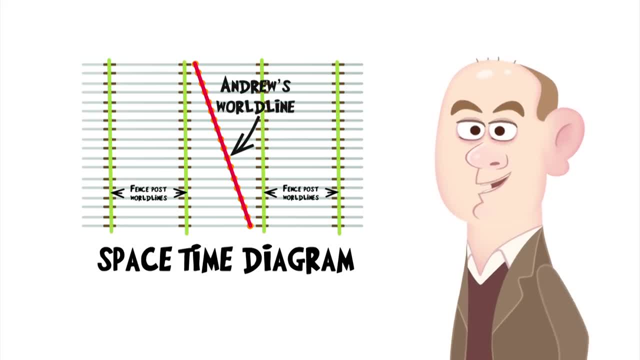 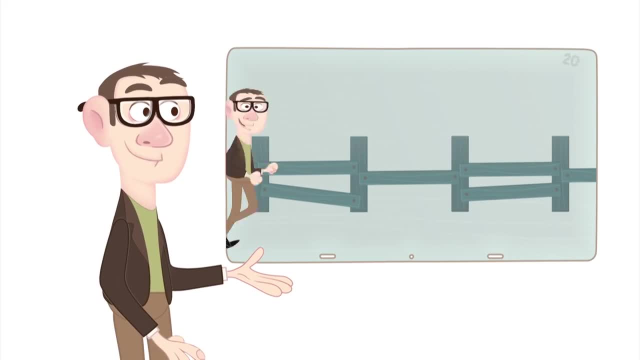 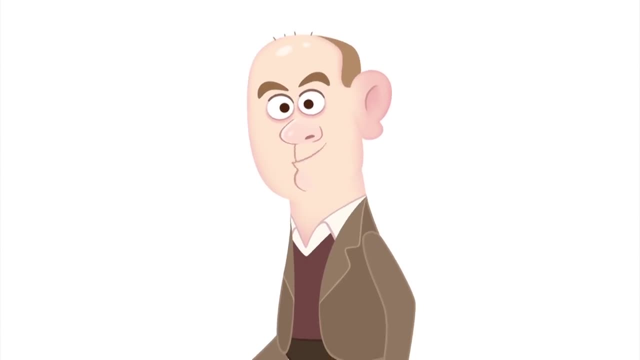 We call the line that represents Andrew's journey his worldline. If I jog instead of walking, I might be able to get past a fence post every second. He's not very athletic. Anyway, when we look at this new flipbook from the edge, we can do the same analysis as before. 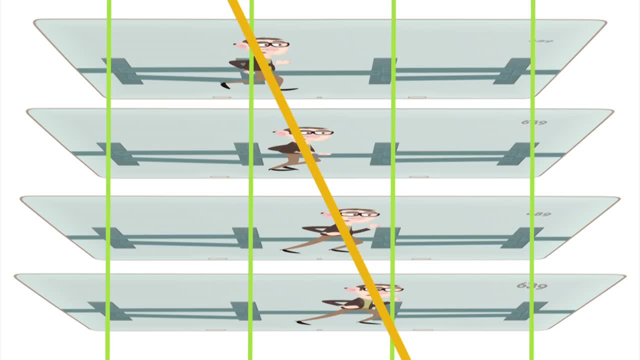 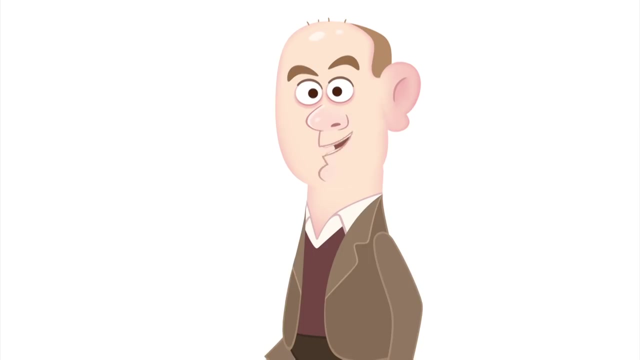 The worldline for Andrew jogging is more tilted over than the worldline for Andrew walking. We can tell he's going twice as fast as before without flipping the panels. But here's the clever bit In physics: it's always good to view things from other perspectives.